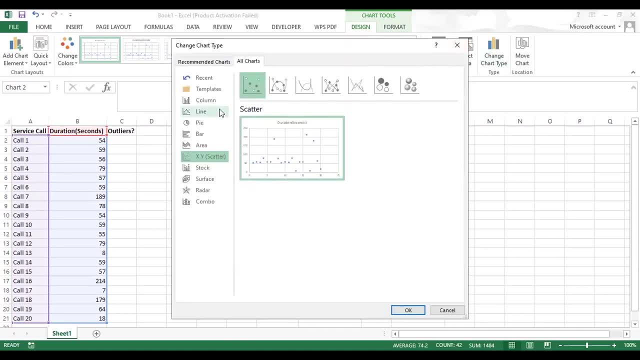 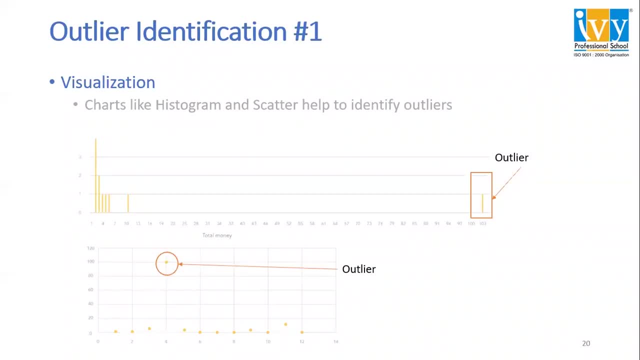 want to change the chart type to say histogram. So my chart is going to be: This is how we can do it. Same can be done for histogram, as we can see in this chart that an outlier will be placed somewhere very outside the charts. Let's move to outlier identification. two Outlier identification: 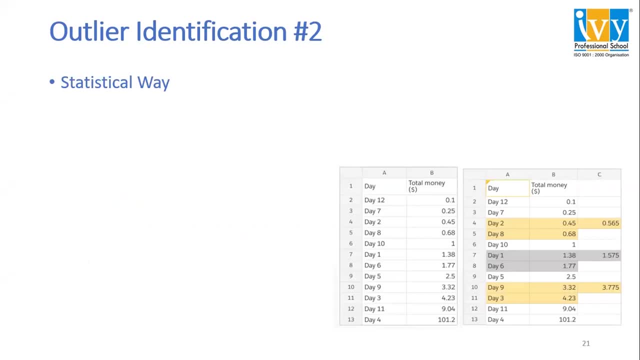 two. So there's a very statistical way of identifying the outlier. We need to sort the data, calculate the quartile and have the formula in this place, And we want the inner and outer fences, Which we call lower and upper bound. Lower bound formula is this: This is the upper bound formula. 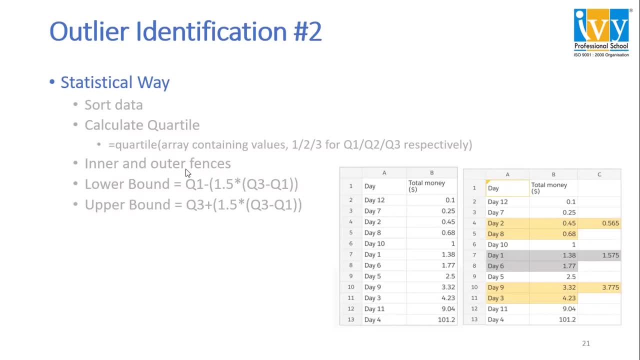 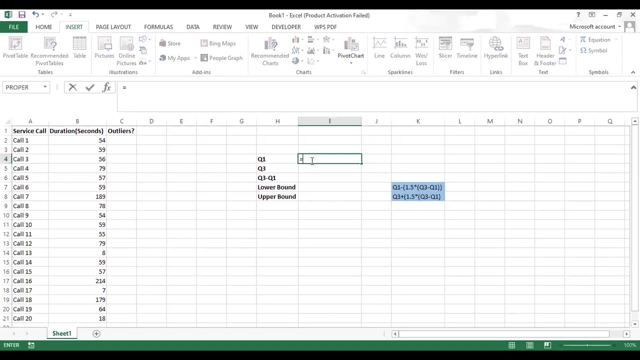 And this is how we can find the outlier. So let's work on the same data set And this is our data set And we want Q1.. Q1 will be basically Formula, for Q1 will be quartile of this whole range and fix it, And the first quartile that is going to be Q1.. Same goes for 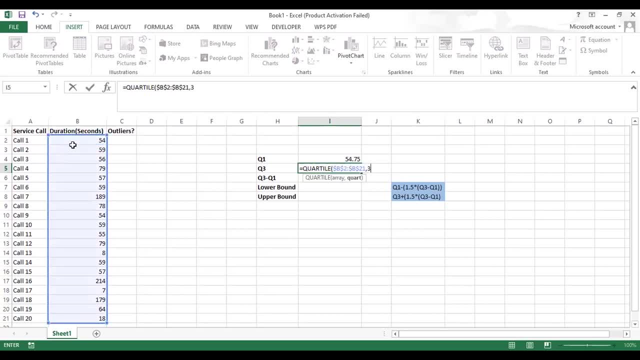 Q3.. The range will be same and quartile is 3.. I want a difference between Q3 and Q1.. So which is going to be is equal to Q3 minus Q1. That gives me 23.5.. Now the formula for lower bound. We say: 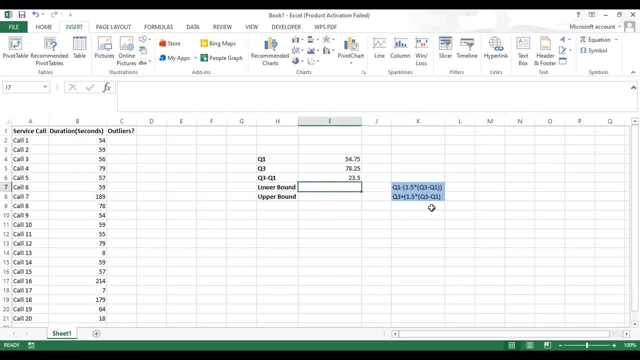 the inner fence and outer fence, which is upper bound, is given here respectively for your reference. So let's just write it. So we want the Q1, which is this minus Q1.. In the bracket, I want 1.5 into Q3 minus Q1, which is 23.5 is equal to 19.5.. 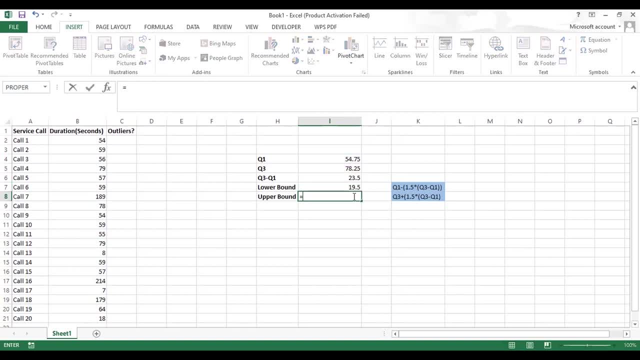 The same thing we want for the upper bound. with the different formulas, It's going to be Q3 plus. we have 1.5 into Q3 minus Q1.. 113.5. now we have to check an outlier based on the lower and the upper bound, the formula which